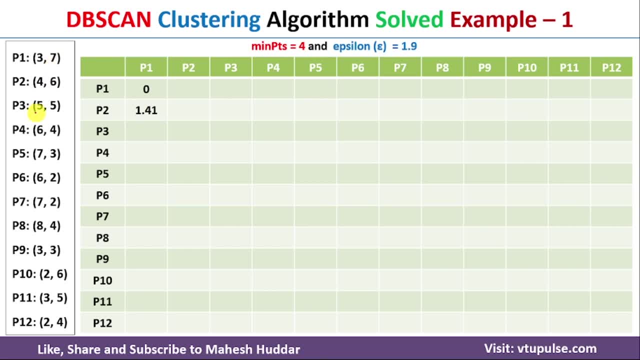 is nothing but x1. y1, in this case is 3 comma 7. x2, y2 is 5 comma 5 here. that is nothing but square root of 5 minus 3 bracket square, plus 5 minus 7 bracket square here. once you solve that, 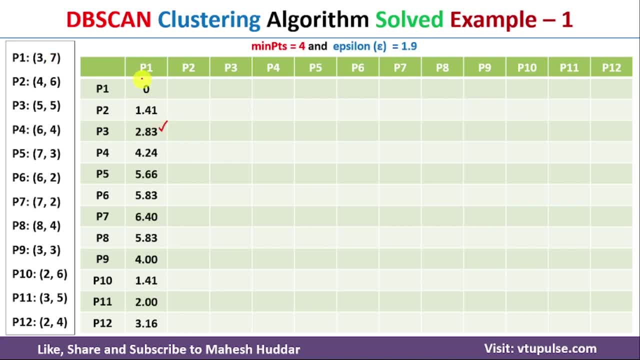 equation, you will get the distance as 2.83. similarly, i need to calculate the distance from p1 to p4, p5 and so on here, once you calculate the distance from p1 to all other data points, next thing is to calculate the distance from p2 to other data points. now there is no need to. 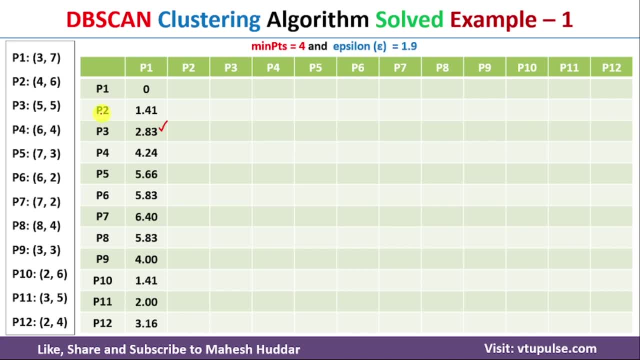 calculate the distance from p1 to p2 to p1, because we have already calculated the distance from p2 to p1. that is equivalent to 1.41, so this is not required to calculate here. next, p2 to p2: that is equivalent to 0. now we calculate the distance from p2 to p3. this is: this is p2 and this is p3. 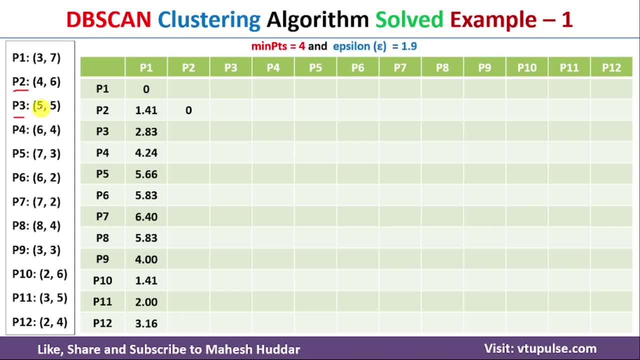 so the square root of x2, that is 5, x1 is 4, so 5 minus 4 bracket square. plus y2 is 5. here y1 is 6, so 5 minus 6 bracket square. so once you solve this equation you will get the distance as 1.41. similarly, we need to calculate the distance from: 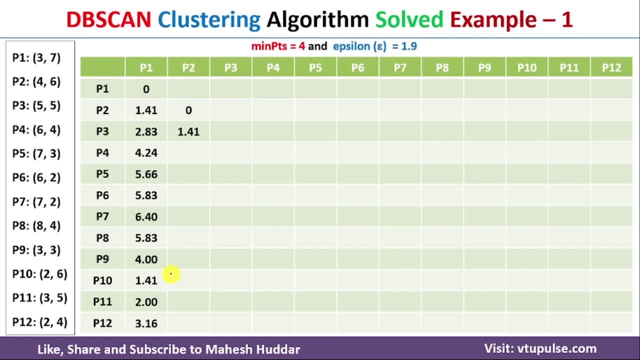 p2 to p4, p2 to p5 and so on. once you calculate the distance from p2 to all other data points, we need to calculate the distance from p3 to all other data points, and so on. so this is how the distances look like once you calculate the distance from p1 to p12 to all other data points here. 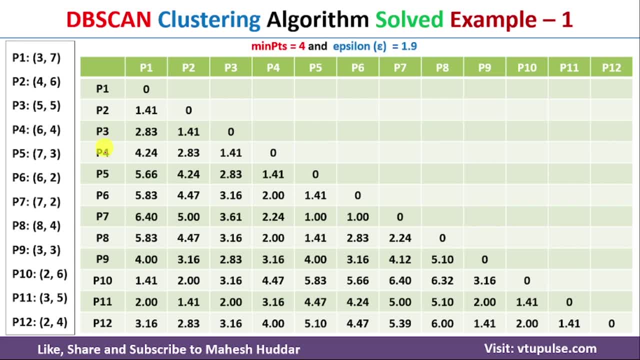 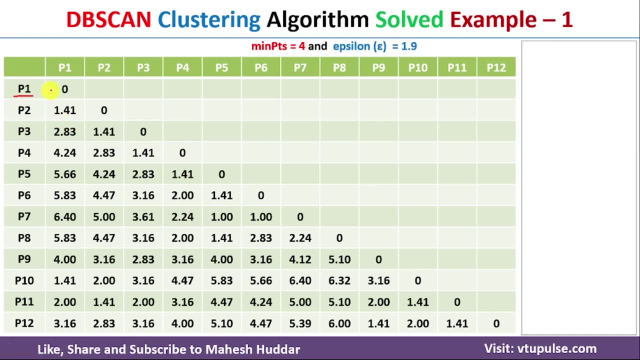 now, once you calculate the distance from one data point to all other data points, the next question comes in front of us is to identify the nearest data points for each of these 12 data points. so these are the distances we have already calculated from p1. we will try to identify. 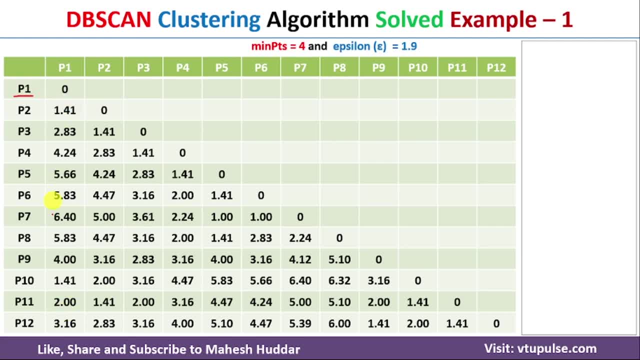 the nearest data point. so first we will start horizontally and then we will start vertically here. so in this case horizontally we have p1 to p1 distance that is equivalent to 0, so p1 will be a part of p1 here. now we will start vertically here, from p1 to all other data points. we will try to find the distance. 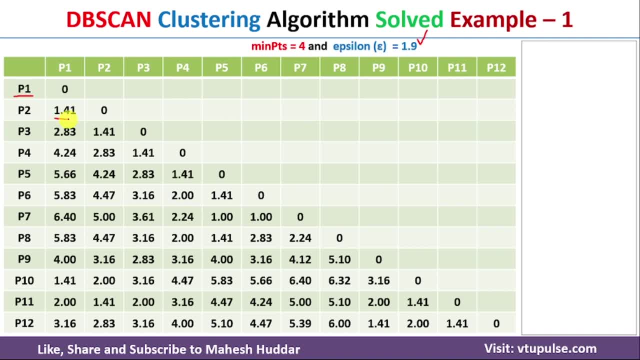 which is less than 1.9 here. so if you look at here, this 1.41 is less than 1.9 and this 1.41 is less than 1.9 here. the meaning of this one is p2 and p10 are nearest to p1 here. so that is what i have. 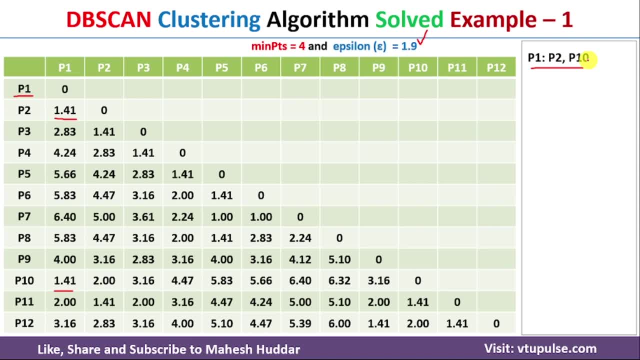 written here to p1, p2 and p10 are nearest in this case. now we will start with p2. as said earlier, we need to start horizontally first and then we need to check the minimum distance. that is less than 1.9. again, 1.41 is less than 1.9. the meaning is: p1 is nearest to p2. here p2 to p2 is: 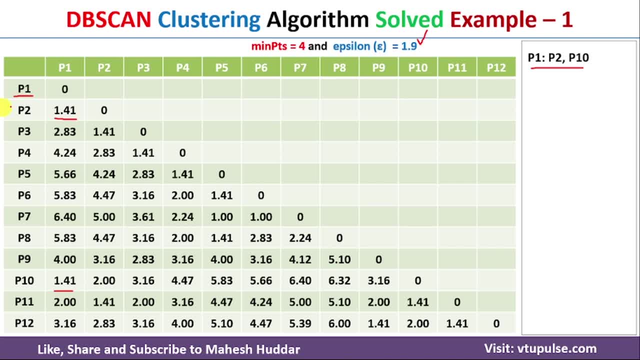 0. the meaning of this one is p2 is nearest to p2. once you are done with horizontally, we need to start with vertically. we need to check the minimum distance. this is the one more minimum distance we have. that is 1.41, which is less than 1.9. if you look at other values again, we have 1.41, which is 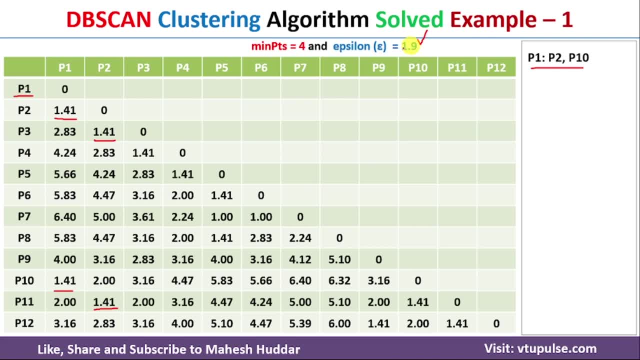 more value. that is, 1.41 is less than 1.9. here. the meaning of this one is to this particular p2. p1 is the nearest one, as well as p3 is the nearest one and p11 is the nearest one. so that is what i have. 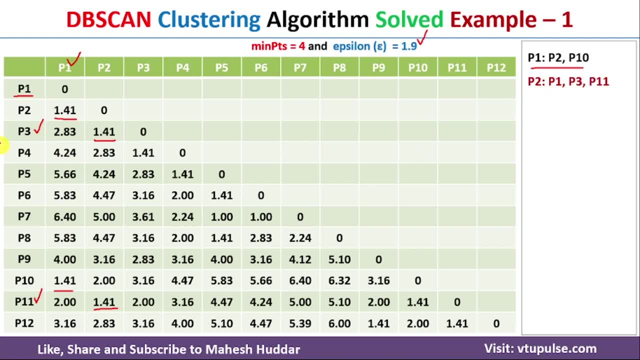 written here. so once you are done with p2, we will start with p3. for this particular p3, horizontally this 1.41 is less than 1.9. the meaning is p2 is nearest. now we will start with vertically, in this 1.41 here, which is less than 1.9- we don't have any other data points- which is less than 1.9. the 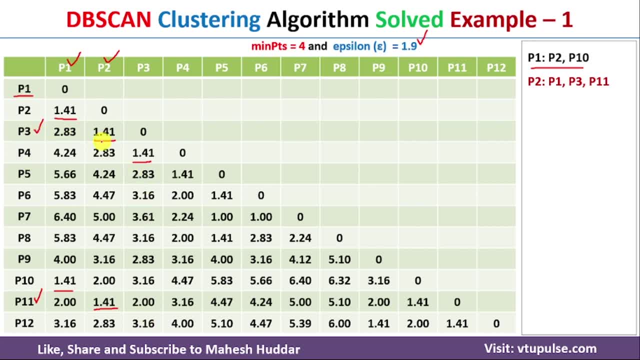 meaning of this one is for this particular p3, p2 is the nearest one, as well as p4 is the nearest one, so p2 and p4 are the nearest one. now we will continue with p4. for this particular p4, horizontally this 1.41 is less than 1.9, so p3 will be nearest value. vertically, if you look at this p4 column, we 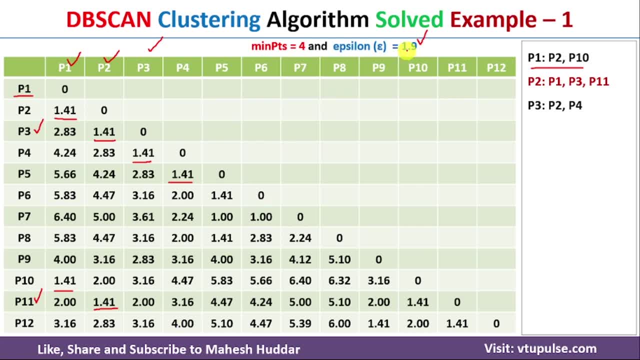 don't have any value which is less than 1.9, which indicates that for p4 this p3 is the nearest one and p5 is the nearest one here. similarly, we need to do it for p5 horizontally. if you look at here, this 1.41 is less than 1.9. that means p4 is nearest to p5. that is the first one. and if you 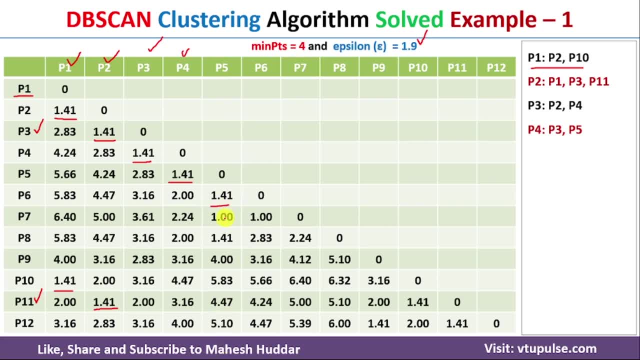 look at this p5 column: 1.41 is less than 1.9, 1 is less than 1.9. 1.41 is less than 1.9, 1.41 is less than 1.9. so for p5, first one is p4, that's the nearest data point. p6, p7 and p8 are also nearest. 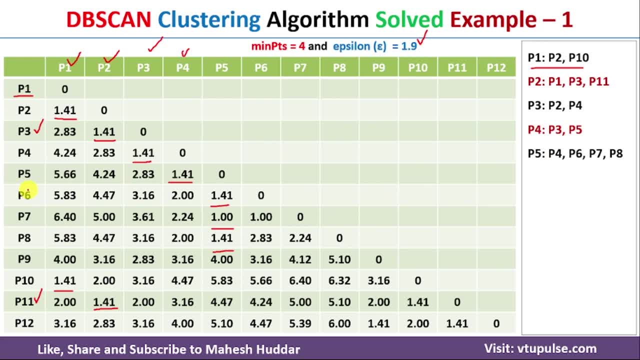 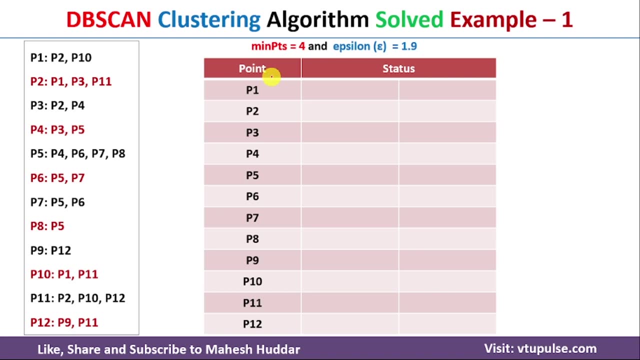 data points over here. with the same note, we need to calculate the nearest data points for p6, p7, p8 and so on. so once you find the nearest data points looks something like this: once you calculate the nearest data points for each of these 12 data points, the next step is to identify the core. 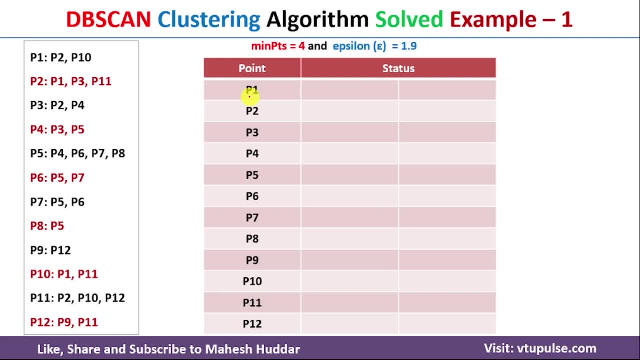 border and noise data points. so I will start with this particular p1. now for p1. we have two nearest data points, that is, p2 and p10. so total number of data points in this case is including p1. we have three, but three is less than. 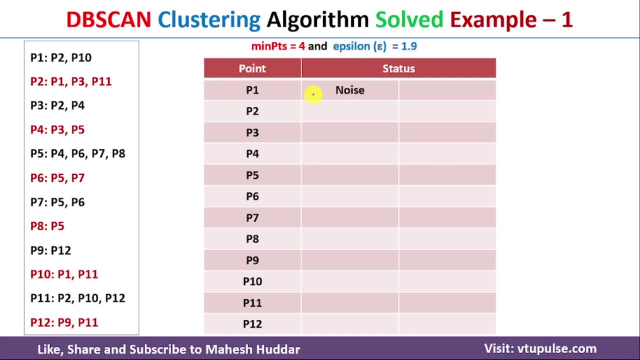 minimum number of points, that is four. hence this particular p1 is called as a noise here. now we will go with p2 including p2. we have four data points here. four is equivalent to four. that is minimum number of points. hence it is called as a core data point. similarly, p3 and p4 are the noise. 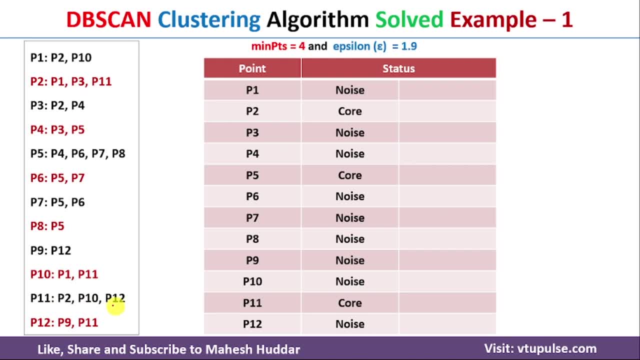 here, p5 is the core and then p11 is a core, because we have four data points remaining. all are noise in this case. so we got one p2 core data point, p5 core data point and p11 core data point here now, once you identify core and noise data points, next we need to check whether any of these noise 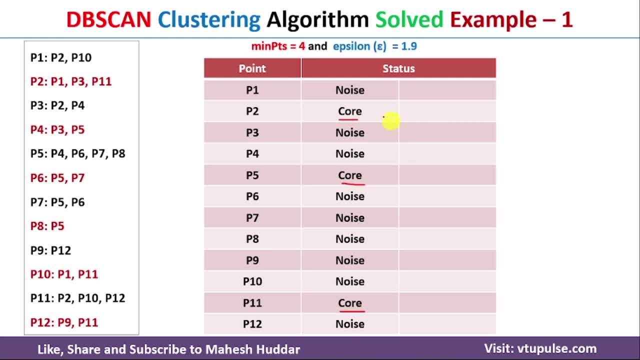 data points are border data points. that is nothing. but sometimes this particular p1 is a noise right now, but p1 may be a border data point. so we need to check whether any of these noise data points are border to the clusters or something like that. so in that case we need to identify whether this 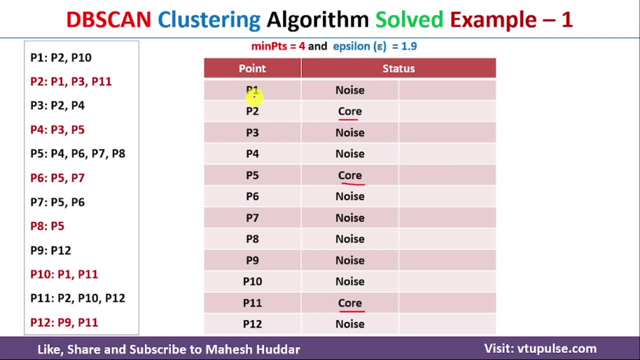 noise data points or borders or what. so i will start with again p1, because p1 is a noise here. now, if we want to say that p1 is a border data point, this p1 should be a part of any one of the core data points. so in this case, p2, p5 and p11 are the core data points if p1 is. 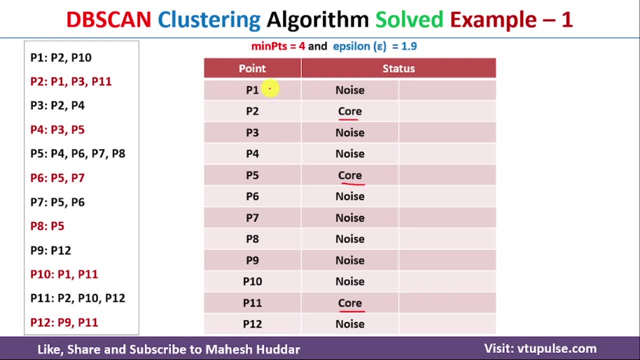 the part of any of this particular core data point. it will be a border here. now i will go with this particular p2. p1 is, you can say that, a part of this particular core. hence it will be called as a border in this case. now i will consider p3. p3 is a part of, again, the p2's core data point. hence 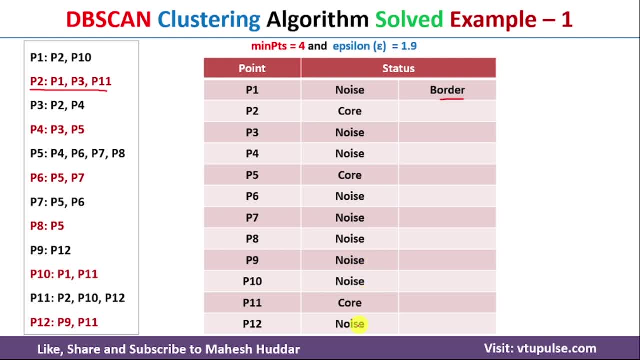 it is also called as border. similarly, we need to check for each of these particular noise data points and then we need to write the border over here. once you've done this particular thing, you can notice this particular p9- p9 remains a noise data point. you can see this particular p9- p9 remains. 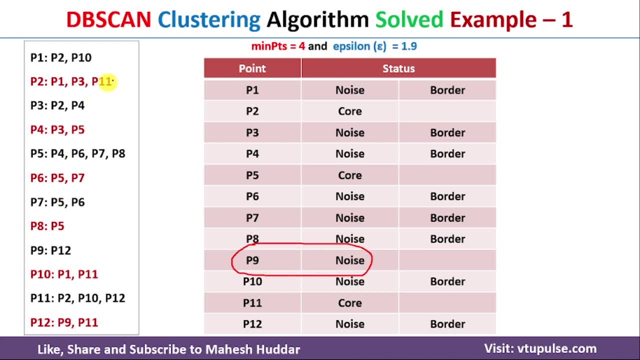 here. the meaning of this one is p9 is not a part of any of this particular core data points over here. so in this case we have p2 and then p5 and p11 as the core data points. the meaning of this one is we will get three clusters centered at p2, p5 and p11 over here. we will try to draw those. 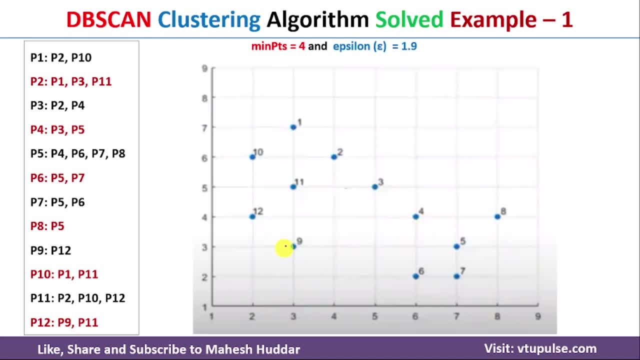 particular clusters. now, first, i have drawn this particular data points on two dimensional space. here this is the data point one is here data point two, three, four and so on. once you draw this particular thing, we need to draw the clusters. the first cluster is with respect to a core data. 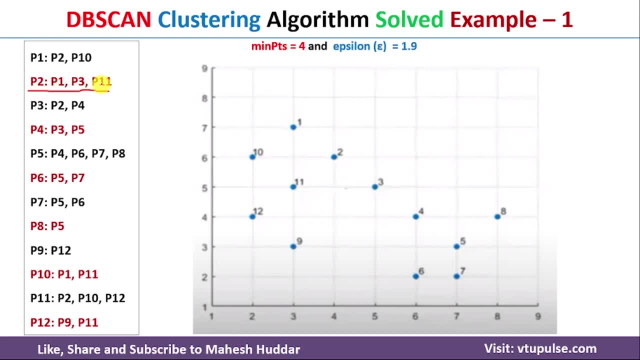 point p2. p2 will be the center here and the remaining three data points will be around this particular p2 here. what are the data points? p1, p3 and p11? so this p1- p2 is over here: p1, p3, p11. 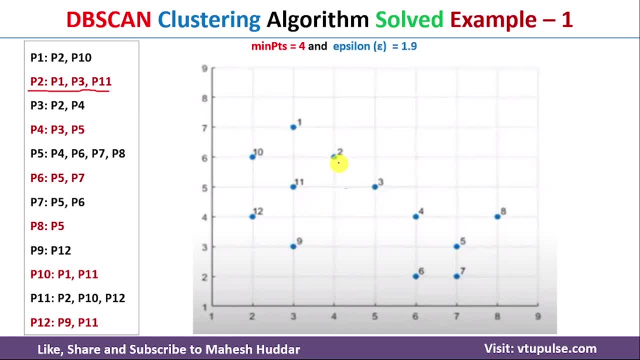 are the other data points in this particular cluster. so once you draw that particular cluster it looks something like this: so this is the data point: p1, p3, p11 and p11. are the other data like this? coming back to the second cluster with respect to core point, p5, p4, p6, p7 and p8 are. 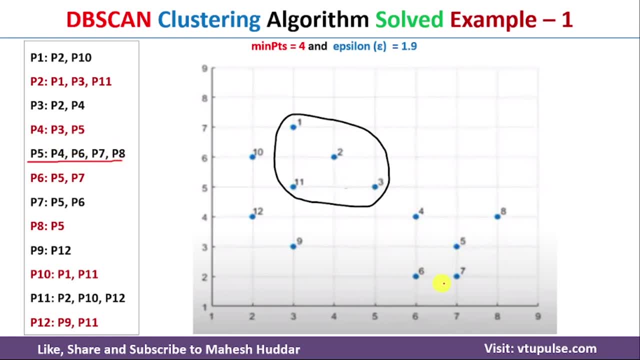 another data points in this particular cluster. so p5 is the center here. around this thing, we will get the four data points here. so once you draw the cluster, it looks something like this: coming back to the last cluster, with respect to p11- core point, we have p2, p10 and p12 here. 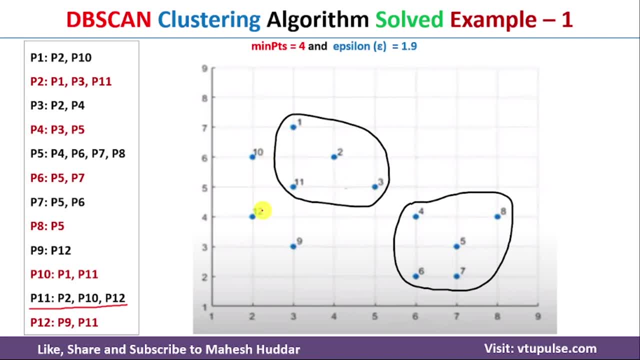 so 11 is the core data point. p2, p10 and p12 are the other data points. once you draw this cluster, it looks something like this: finally, we got three clusters. uh, with respect to db scan clustering algorithm for these 12 data points, they look something like this. so this is how we can apply.